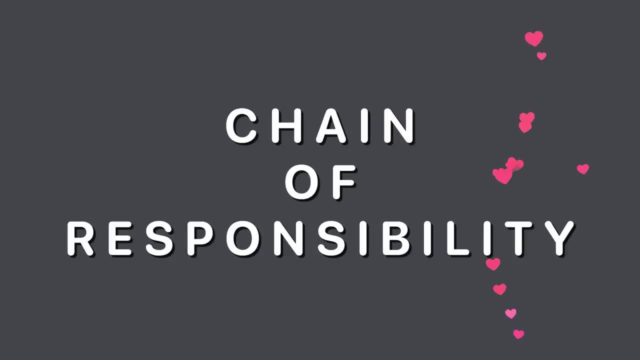 It's not the most popular design pattern, but it's my favorite. If you are new here, like and subscribe, and if you like my videos, let me know. what do you want to see next in the comments? As always, the final code you can find on my Github repository. 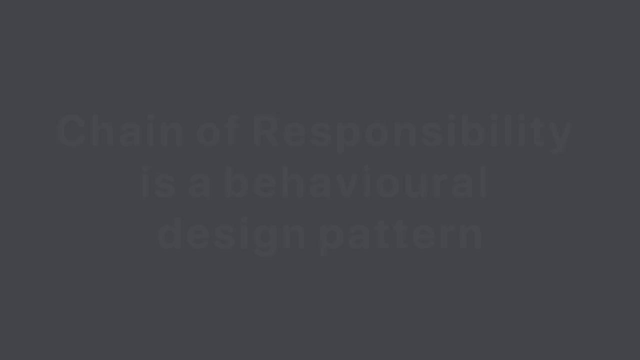 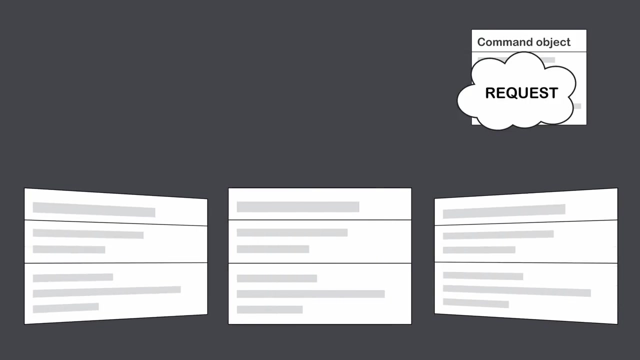 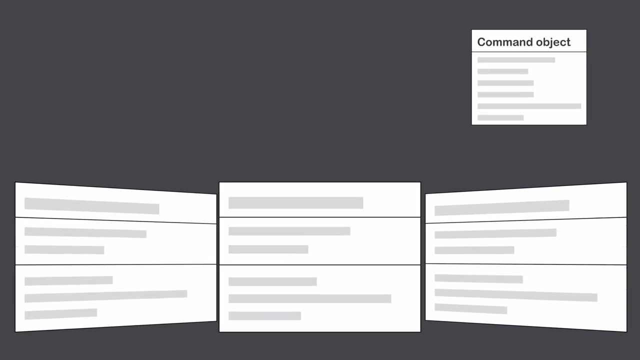 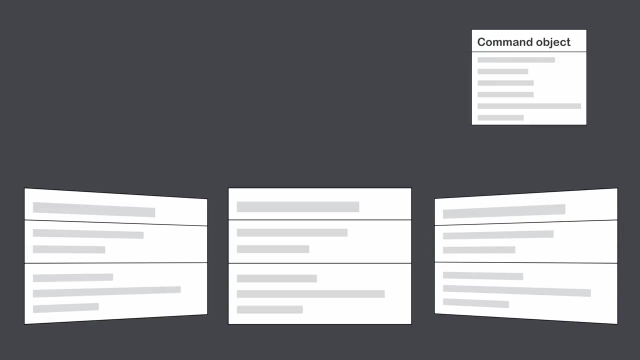 The link you will find in the description. Chain of Responsibility is a behavioral design pattern that lets you pass requests along a chain of processing operations, objects, also called handlers. So this pattern consists of a command object and group of processing objects. Each processing object decides either to handle the request or to pass it to the next processing. 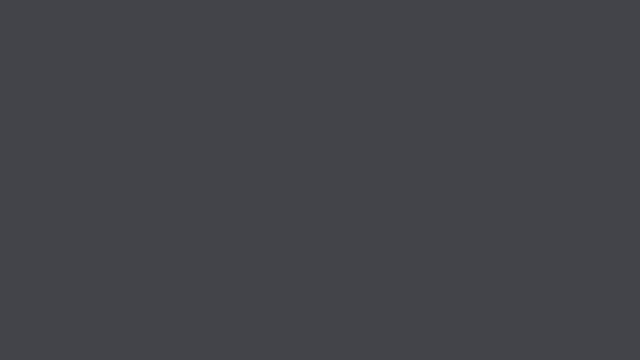 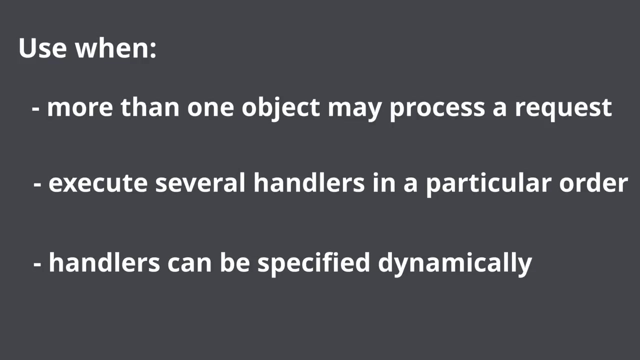 object in the chain. You should use pattern ChainOfResponsibility. when more than one object may process a request, The processing object should be defined automatically. It's essential to execute several handlers in a particular order. The set of objects that can handle a request should be specified dynamically. 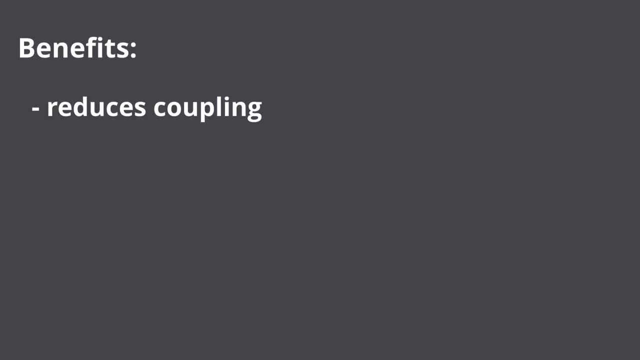 This pattern has following benefits: Reduces coupling. Decouples the sender of the request and its receivers. Reduces complexity of your object because it doesn't have to know the chain structure and keep direct references to its members. Adds flexibility: Allows you to add or remove responsibilities dynamically. 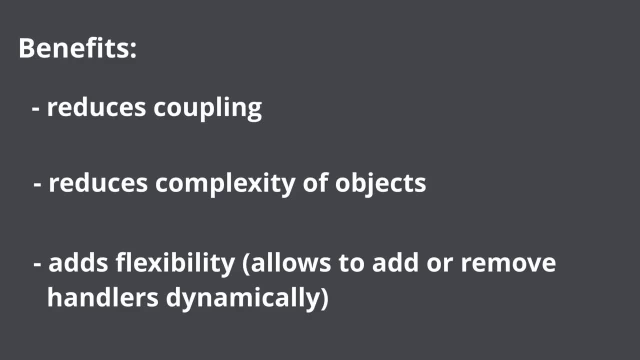 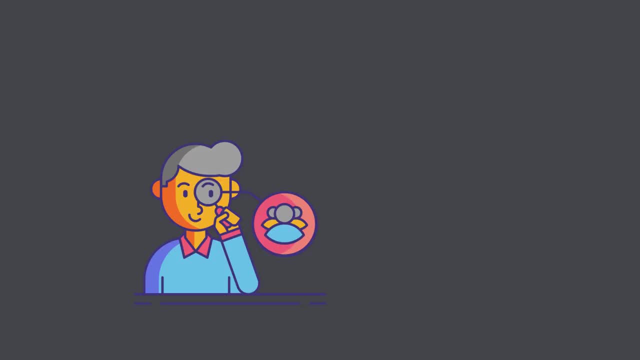 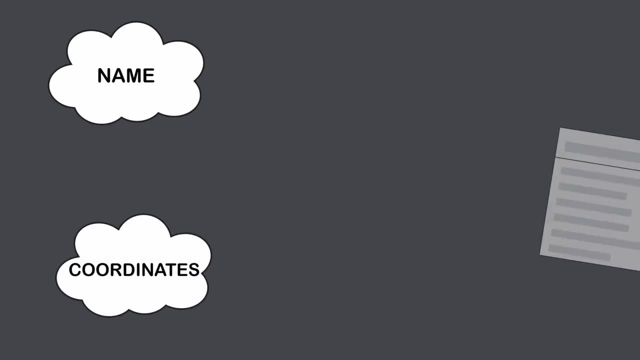 By changing the members or order of the chain. Let's take a look at this pattern with a simple example. Imagine situation when customer wants to get information about some place And for this he provides some input parameters, for example name of this place or its coordinates. 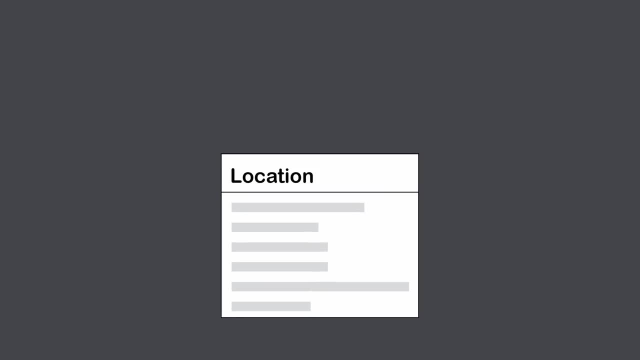 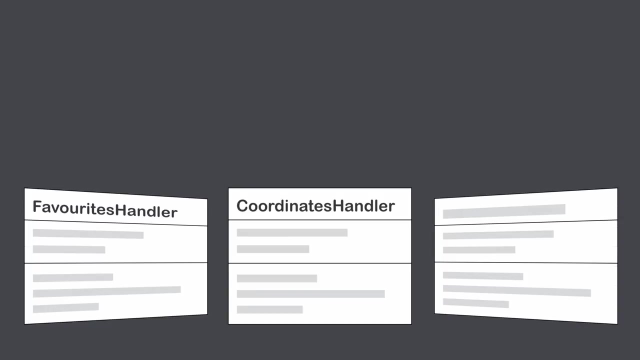 Technically speaking, we need an object location with some set of fields, for example name, street, city, country and coordinates, And there will be several handlers which will process a request. For example, it will be favorites handler, coordinates handler and name handler. 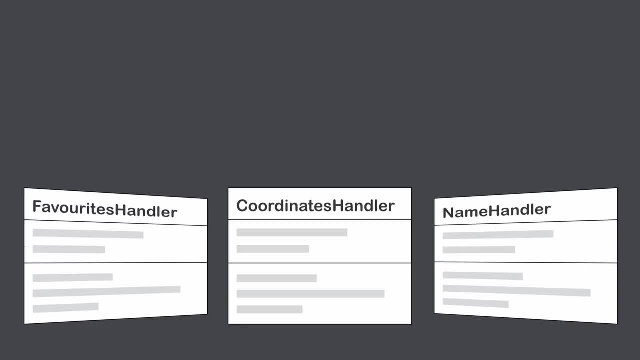 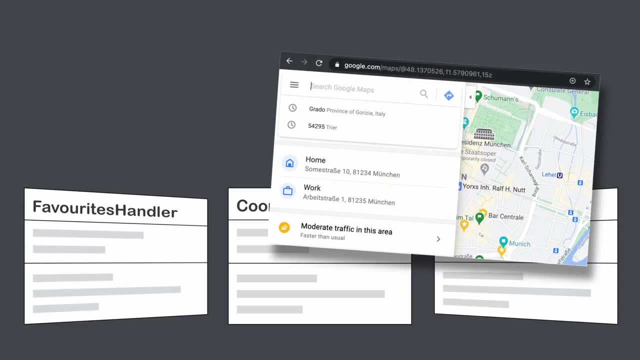 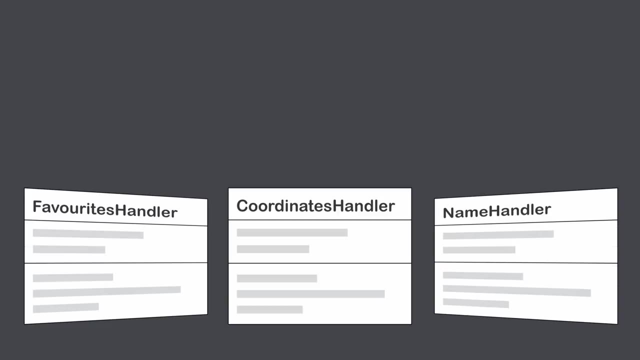 And processing order will be the same. Favorites handler will check customer's favorite places. Imagine it as a shortcut, like in Google Maps Home or work, and behind each name there are coordinates of a real place. Coordinates handler gets location from Google Maps API by provided latitude and longitude. 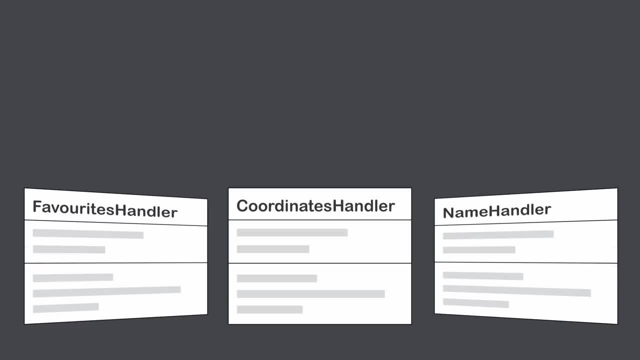 Name handler gets information from OpenStreetMaps API by place name. All these handlers implement the same interface, which has methods setSuccessor and process. setSuccessor is called in order to create a chain process. method is called to execute processing request. 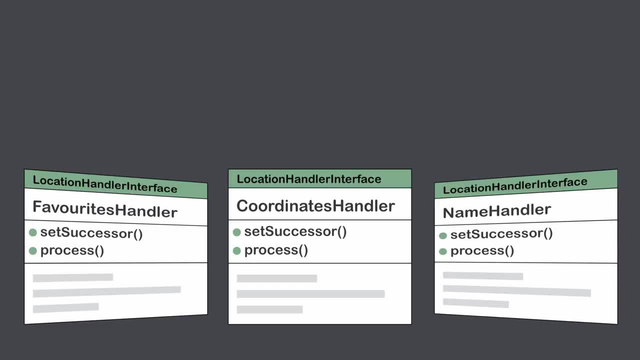 Each handler checks incoming request and decides to process it or not. So favorites handler checks if request has a name and it is defined in a customer list of favorite places. Coordinates handler will process request with latitude and longitude Name handler processes request only when name is present. 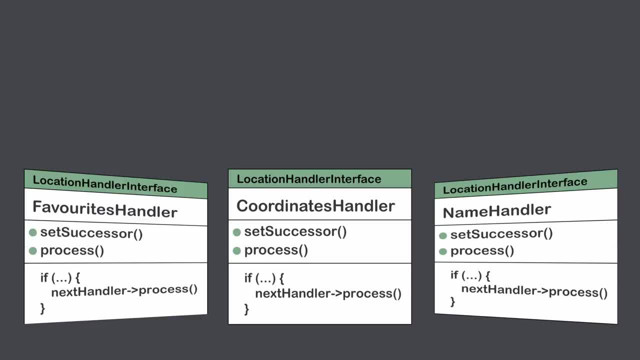 It may happen that no handler can process a request For this pattern. it's totally valid case and you should consider it during implementation. When customer sends a name for a place like my home command object, receives it and passes to first handler from the chain, which in our case is favorites handler. 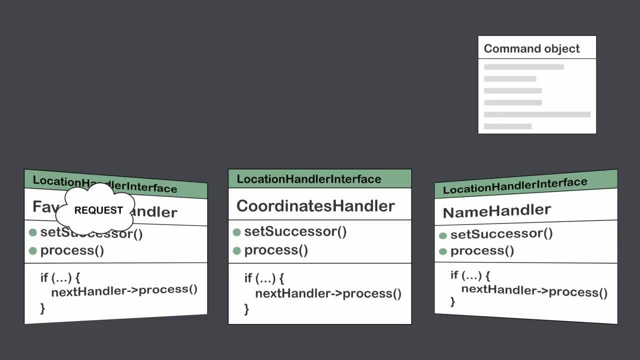 Ok, name is present in the request. so with next step this handler checks if place with such name is defined in a customer's list of favorite places. Let's say it's defined. Handler gets coordinates by name and sets them into request. Then it calls process method of next processing object in the chain. 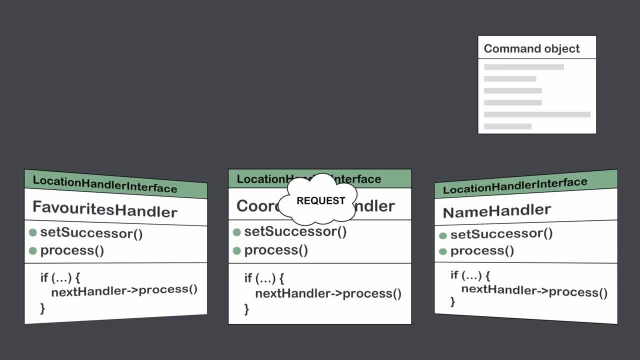 Request contains coordinates, so coordinates handler also can process this request. Handler calls Google and fills all missing information And it calls process method of next handler. The last handler is name handler and it could process a request because name is present, but request already has all information and there is no need to do anything else. 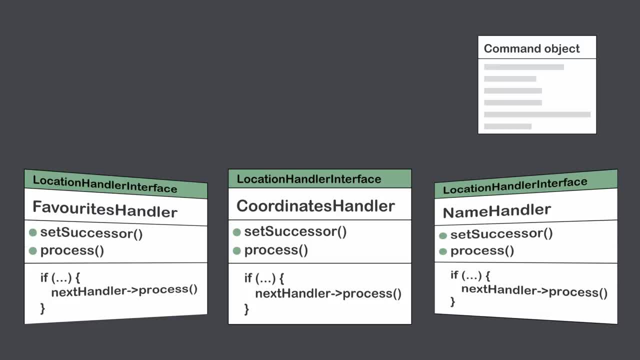 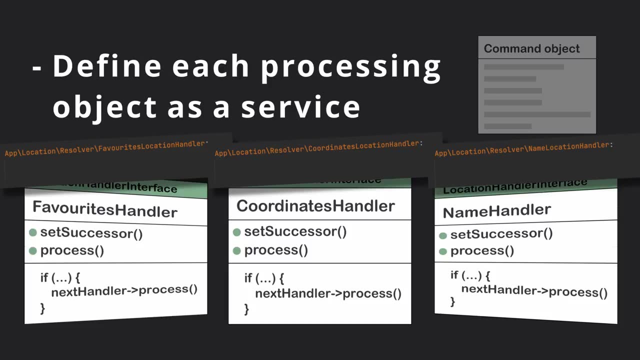 Processing is complete, as there is no next processing object in the chain. To implement chain of responsibility pattern in Symfony application we should perform several steps: Define command object SSL. Define each processing object as a service. Add some custom tag to the service definition, for example location handler. 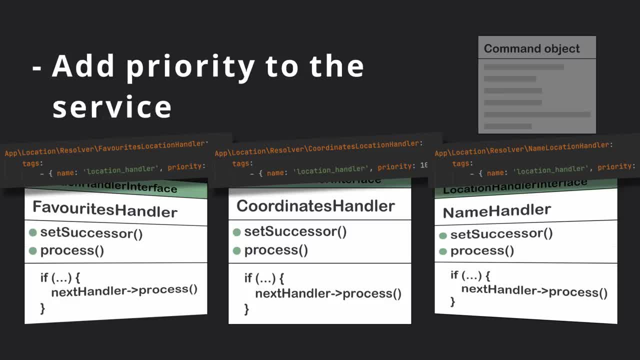 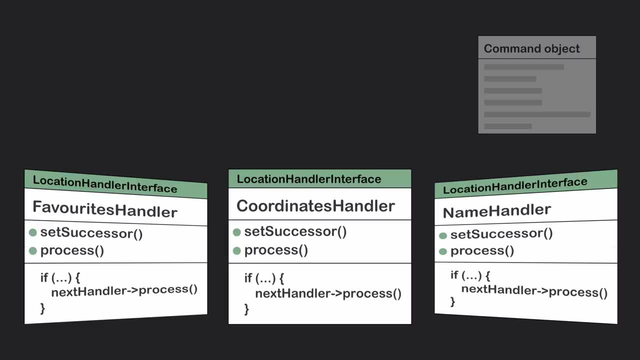 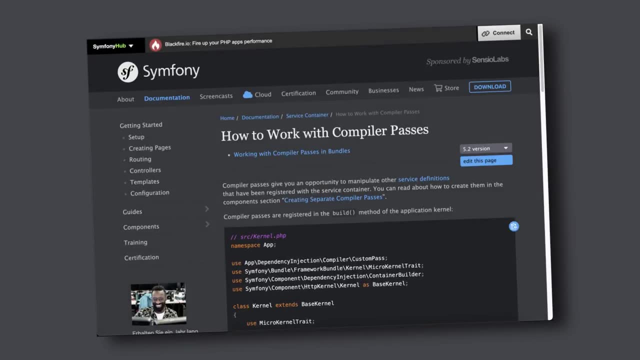 Add priority to the service to set desired order for processing objects. We should write a compiler path to work with service definition before service will be assembled in Symfony container during bootstrapping of application. You can read more information about compiler path in the official Symfony documentation. 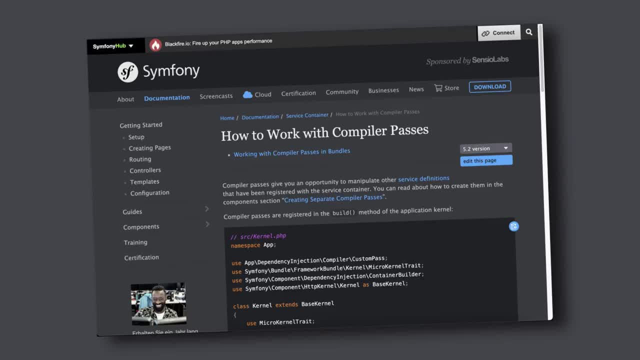 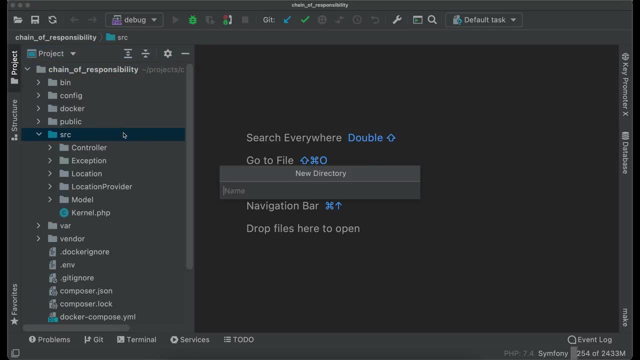 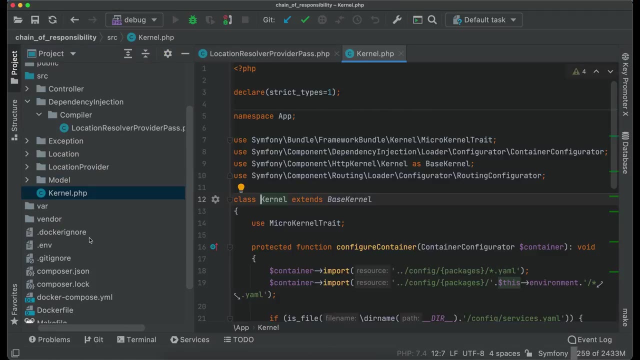 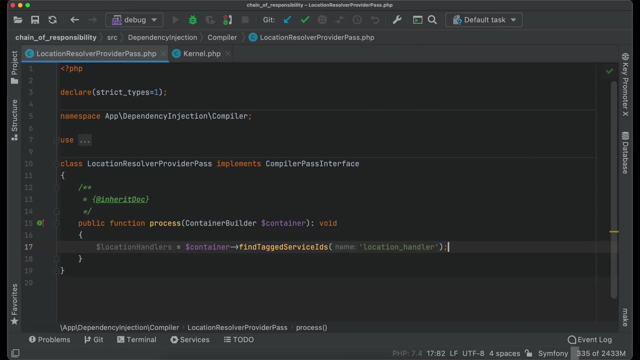 Thanks for watching The link you will find in the description block below this video. Create a new compiler path. Add it to the kernel class. In the compiler path, find all services tagged with our custom tag and sort services by priority. Get first handler from our data source. 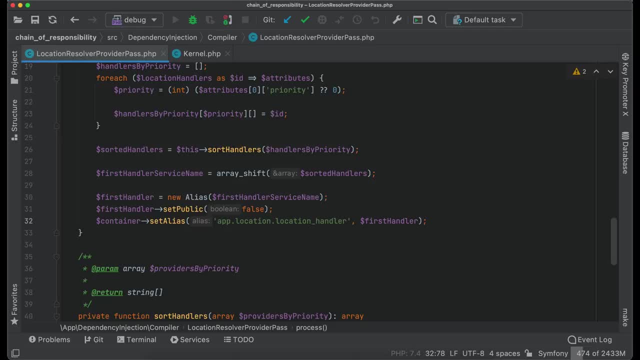 handler from array and create a new alias object with this handler. It means that this service will be accessible for injection via our custom alias. Now iterate through all handlers, get next one and set it as a successor to previous handler. With this manipulation, each handler knows the next one. 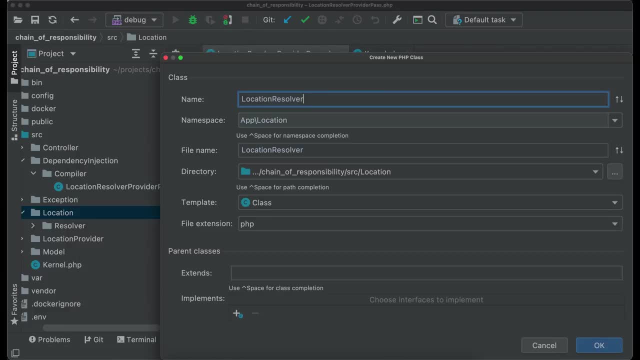 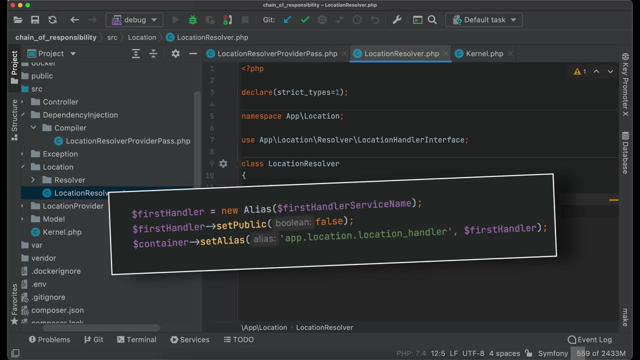 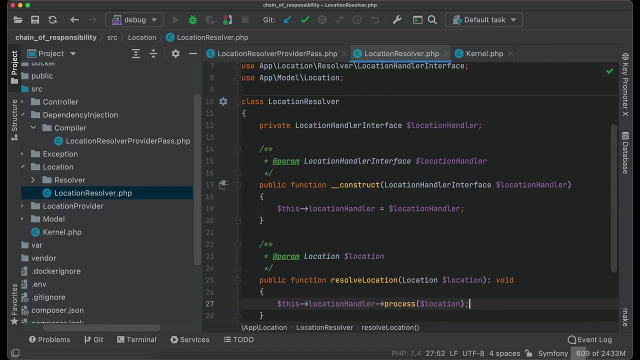 The chain is ready. Create a new class. it will be a location resolver. Inject first location handler there, Remember, we have defined an alias for this service. This class will have public method resolveLocation, which accepts location object and processes it. 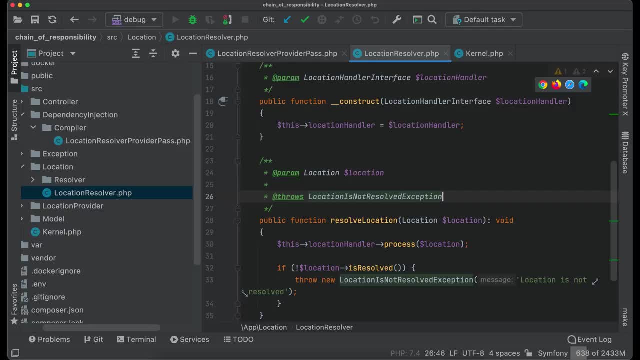 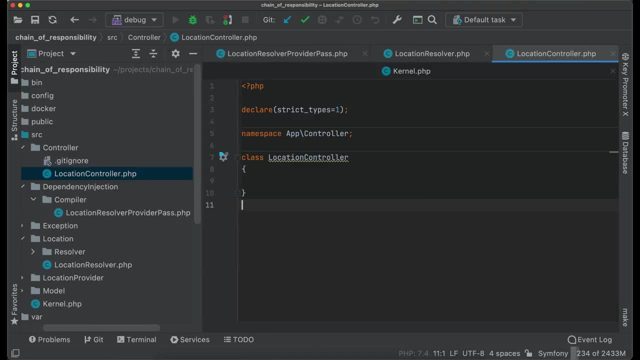 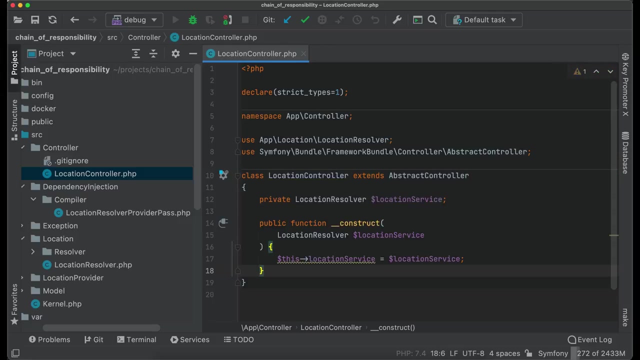 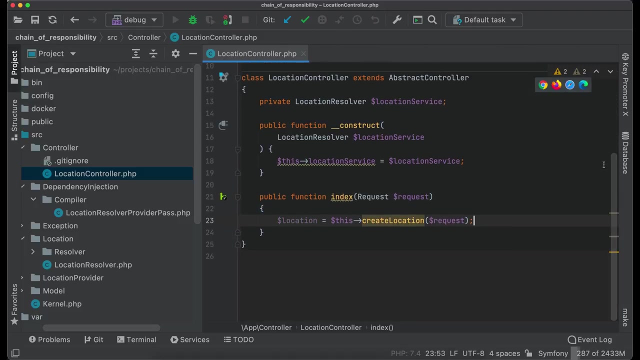 If location is not resolved by any handler, error will be thrown. Now we can test our implementation For this. let's create a controller and inject location service. Define new action. Create location object from request. Ideally, symphony form should be used here, but this is another topic. 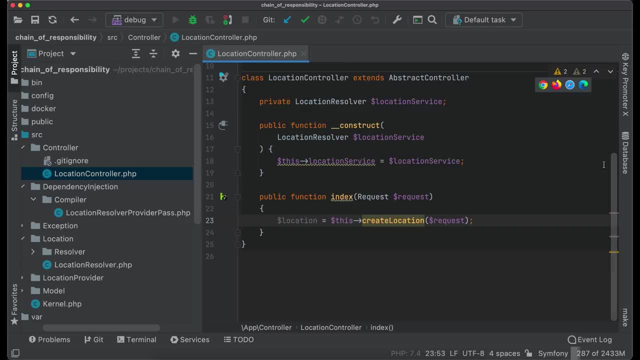 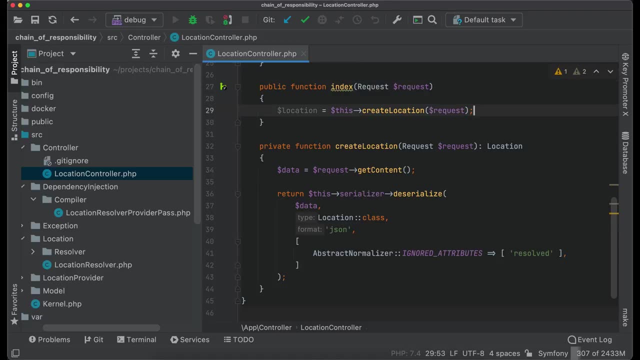 The link to forms tutorial you will find in the info box somewhere on the right top corner. For demonstration purpose, I will use serializer component, So call resolveLocation and pass location. object: Wrap applicationException with httpException And at the end add a new one. 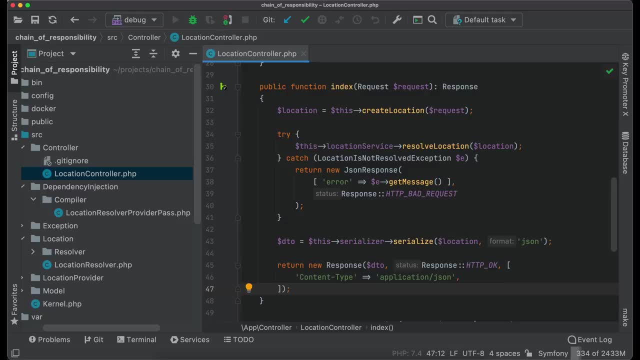 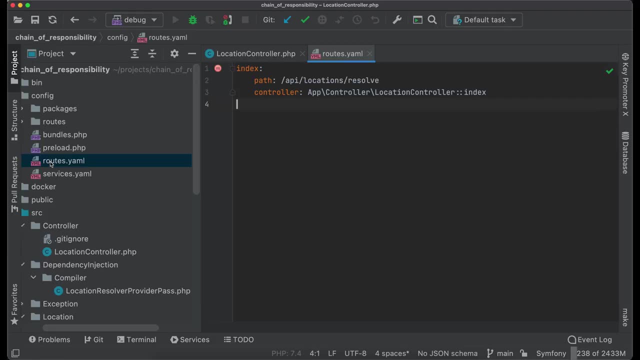 And here we are. Let's start And return JSON response, Define new route And we are ready to test our implementation. By the way, sample project from github with final code is dockerized and has xdebug, so you can easily run it locally and check execution step by step.